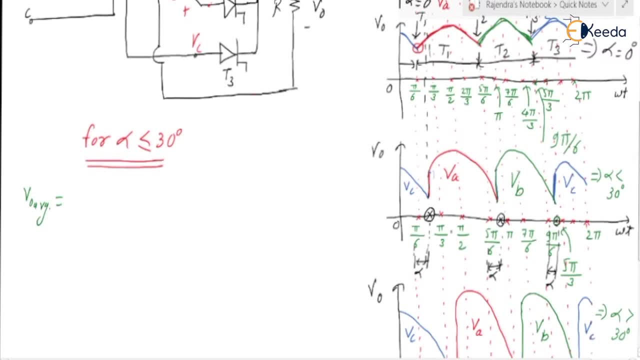 So here, V0, average right in the V0 waveform for alpha, less than 30 degree right, the VA is appearing from: yes, from this instant okay to this instant okay. So here, if you check, can we write this instant, this is pi by 6 and this angle is alpha. 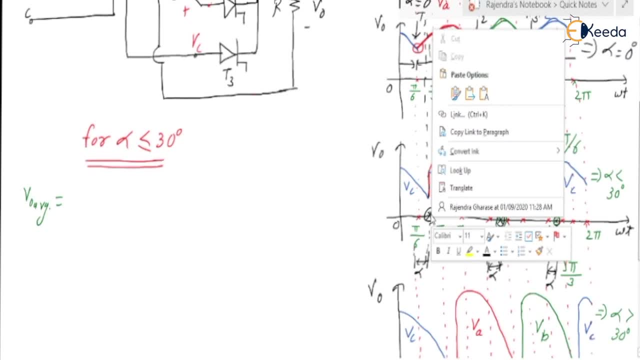 So can we say that this instant is pi by 6 plus alpha? yes, this instant, This is pi by 6 plus alpha. okay, Again, what is this instant? Yes, it is a 5 pi by 6, okay. 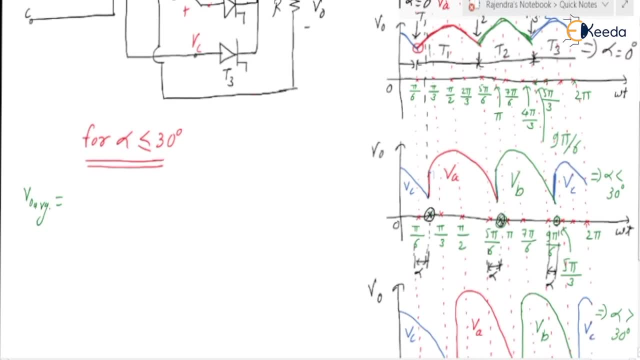 And this indicates the alpha. okay, So it is like a 5 pi by 6 plus alpha. okay, So you can write it as yes and again corresponding to one input cycle in the output where I have the three pulses. okay. 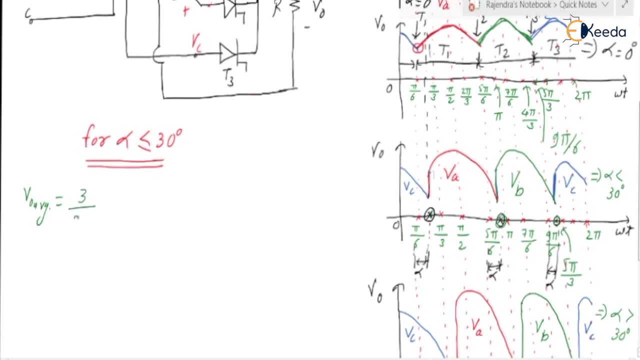 So V0 average is equal to it is 3 by 2 pi. integration from: yes, pi by 6 plus alpha, pi by 6 plus alpha, right? So yes, upper limit is 5 pi by 6 plus alpha. okay, 5 pi by 6 plus alpha okay. 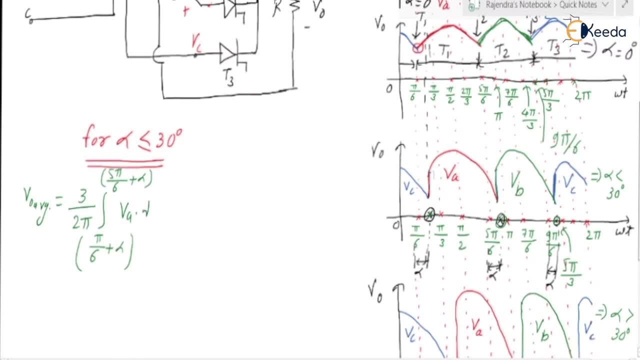 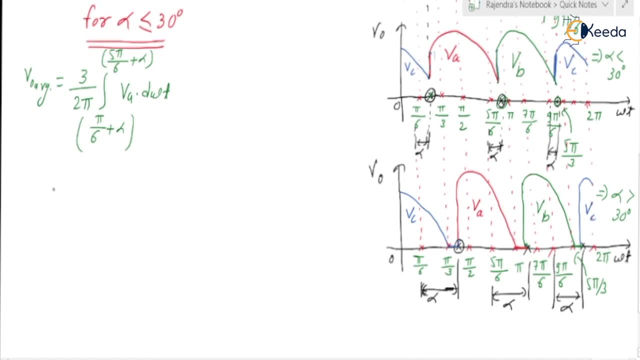 During this interval in the output we are having VA only. okay, So it is a VA into d, omega t. right Again, what is VA? VA is equal to Vm into sine of omega t, So it is equal to: we can write it as a 3 by 2 pi. yes, into integration from pi by 6 plus alpha to. 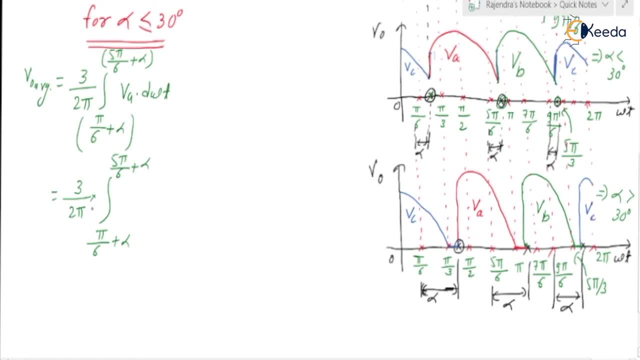 5 pi by 6 plus alpha. yes, What is the VA? VA is Vm into sine of omega t to d, omega t right. So further can we simplify it as: yes, this can be written as: yes, we can write this as is equal to: we can take Vm outside. 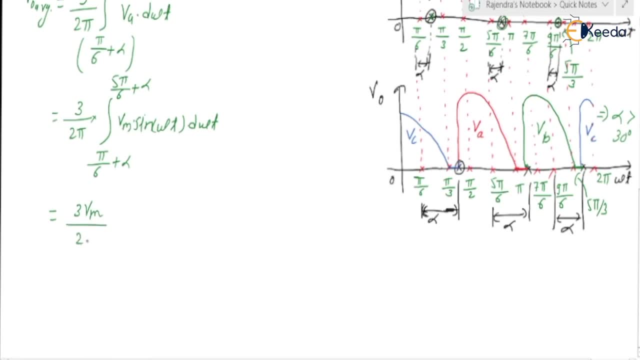 So it is a 3 Vm divided by 2 pi, okay, into yes integration of sine. Again, it is a minus cos of omega t, okay, and the limit is pi by 6 plus alpha to 5, pi by 6 plus alpha, okay. 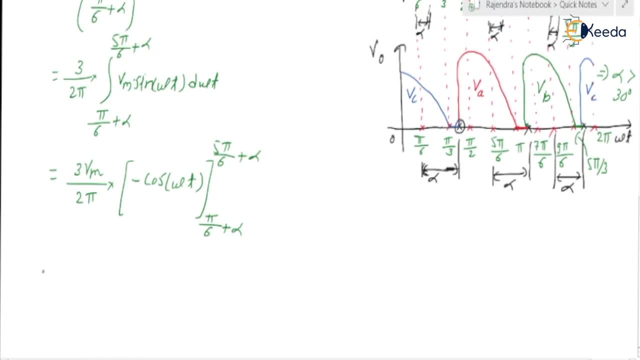 So therefore, if we put the limit- yes, it will be equal to 3 Vm by 2 pi- into yes, we can write it as a minus cos of 5 pi by 6 plus alpha, plus cos of 5 pi by 6 plus alpha right. 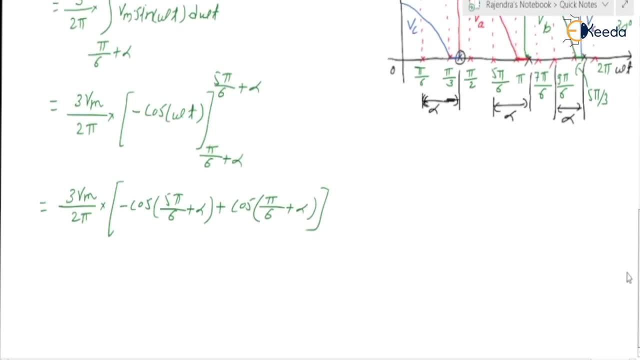 So further, can we simplify it as cos of alpha plus beta? yes, we can write, so I am writing directly here. So it is a 3 Vm divided by 2 pi. okay, into: yes, this can be written as. yes, it is a cos of. 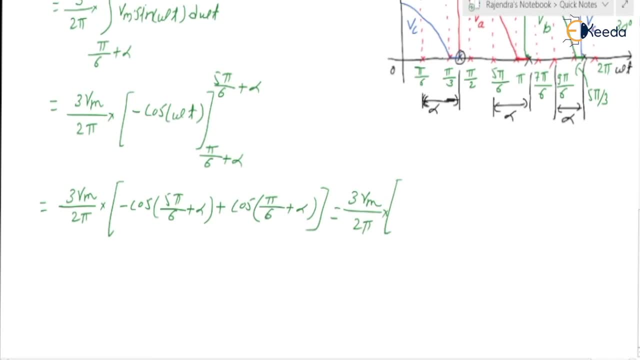 alpha plus beta. okay. so cos of alpha plus beta. and this is also cos of alpha plus beta, okay. What is the cos of alpha plus beta? Yes, it is cos A, cos B, right, minus sine A sine B. okay. cos A, cos B minus sine A sine B, okay. 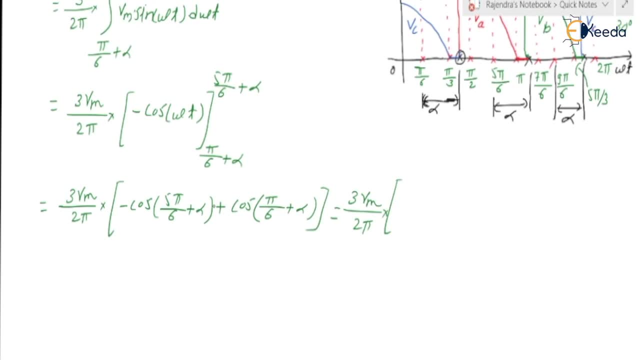 So it is a cos of 5 into 118 divided by 6, so it is a minus 0.86, that minus and this minus it will be, so it is a 0.86, into cos alpha minus sine A, sine B. okay, yes, it is a 0.5, right. so it is minus 0.5 here. okay, into sine alpha, right. 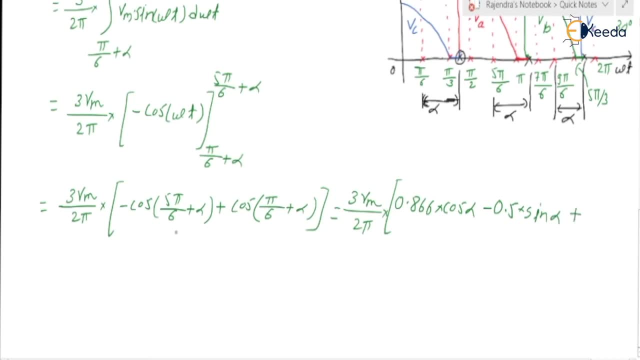 this is the one term- plus cos of pi by 6, plus alpha, cos A, cos B. yes, so it is a 0.866, 0.866, into cos alpha, right. right. sine of pi by 6 is a 0.5, okay. so plus 0.5 into sine alpha, okay. 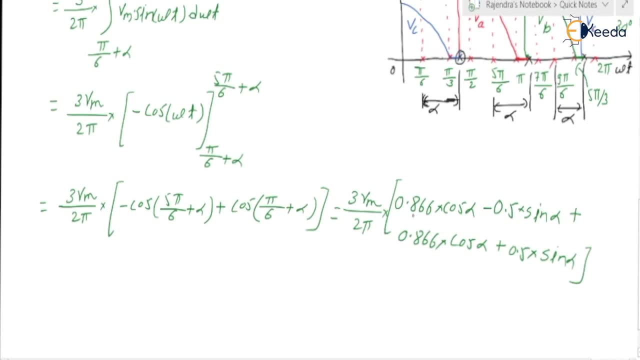 so it is a cos A plus B. okay, cos A cos B, right. So it is a cos of pi by 6 minus sine A sine B. okay, next, sine of 5. pi by 6, 0.5, okay, so 0.5 into sine alpha okay. 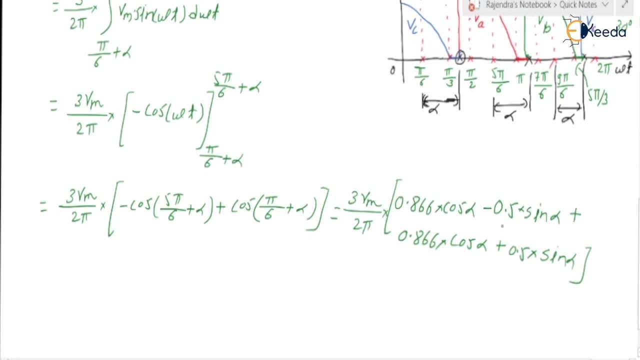 So next. so from this 0.5 sine alpha, 0.5 sine alpha, it will get cancelled. okay, so this can be written as 3 Vm divided by 2 pi and 0.866 cos alpha plus 0.866 cos alpha. okay, so this is. this can be written as 3 root 3,. 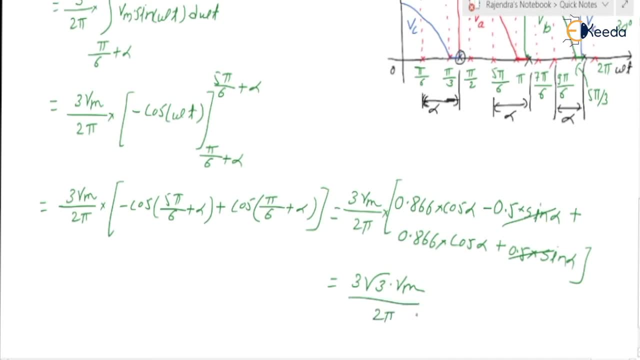 2 Vm divided by 2 pi into cos, alpha. this is what the V0 average we are having, you know, for omega t, sorry for alpha- less than 30 degree or equal to 30 degree, very, very important expression. okay. 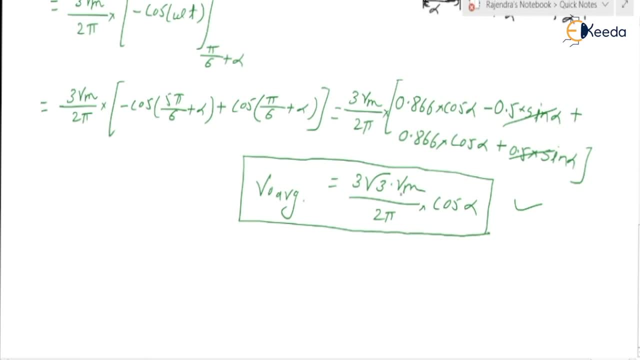 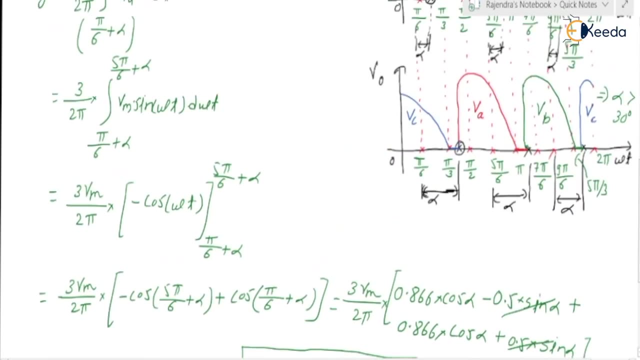 3 root 3 Vm by 2 pi into cos alpha. what is the Vm is the peak value of the phase voltage. okay, vm is nothing but peak value of the phase voltage. so here, if you check vm, that is the peak value of the phase voltage. 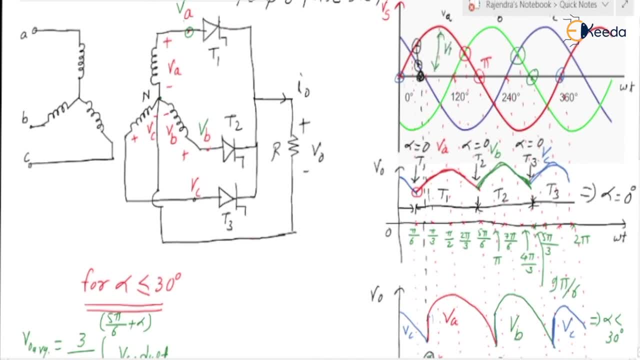 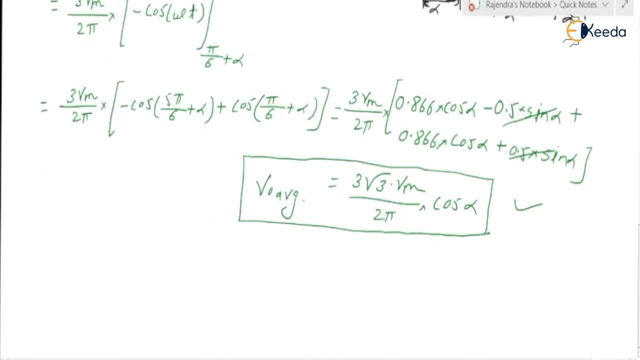 yes, this indicates the vm value. right next, this is the v0 average for alpha less than 30 degree. okay, next can we find the v0 rms? yes, we can write v0 rms. v0 rms- square root of mean of squared value. okay, so it's a 1, 3 by 2 pi. 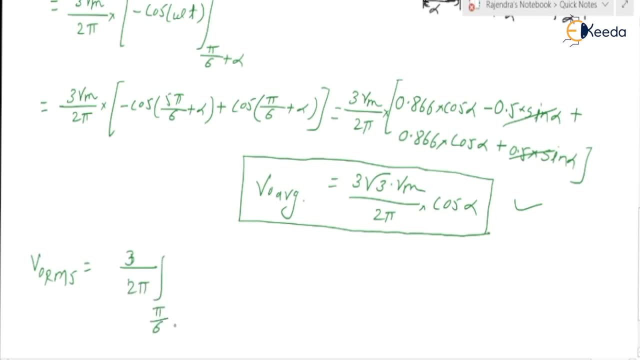 integration from pi by 6 plus alpha to 5. pi by 6 plus alpha. yes, it is vm square, sine square of omega t to d, omega t, the power, 1 by 2 to the power. okay, so therefore, if you check, or can we simplify it? 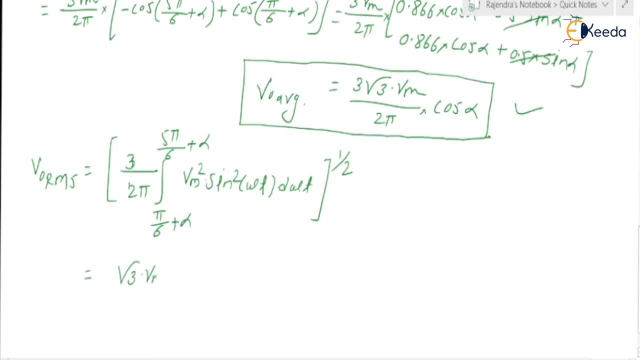 as yes, it is, root 3 into vm squared by 2, 2 pi. okay, into this integration of pi by 6 plus alpha to 5, pi by 6 plus alpha and square can be replaced with 1 minus cos of 2. omega t squared by 2 to omega the power, 1 by 2. 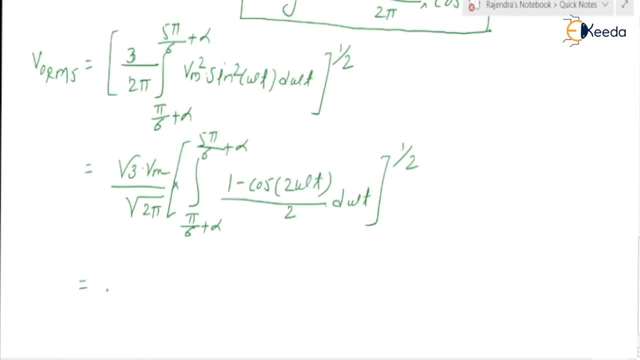 further. we can simplify it as is equal to, as i am taking this divided by 2 also outside, so it will be root 3 into m squared by 2. root pi: okay into s as omega t. okay, minus integration of cos, it is sine of 2 omega t. 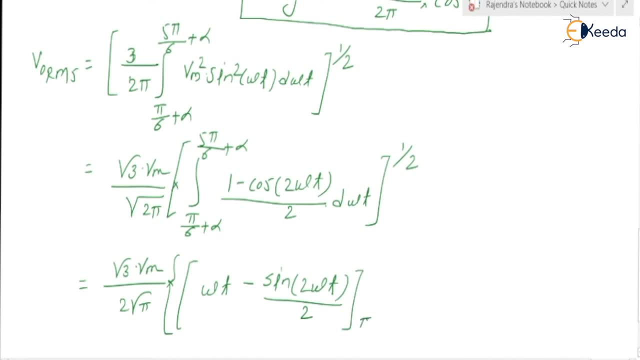 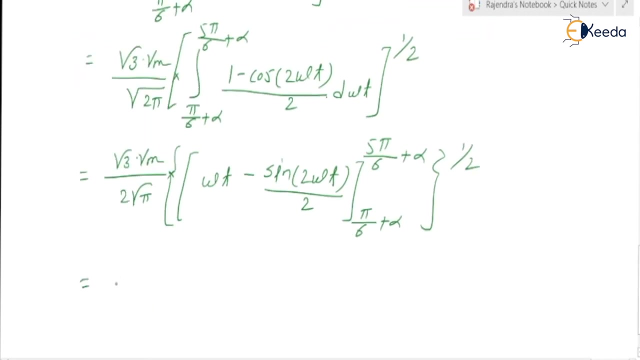 squared by 2, split pi by 6 the alpha to 5 pi by 6 the power 1. further, we can simplify it as is equal to root 3: vm squared by 2, root pi into: yes, this can be written as 5 pi by 6 plus alpha, minus 5 by 6 plus alpha. 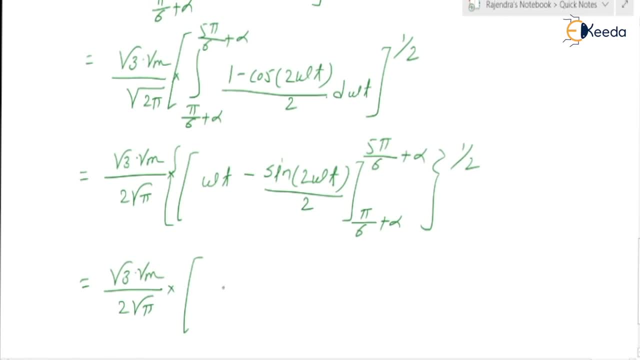 so it is a 4 pi by 6, right? 4 pi by 6. okay, 4 pi by 6 means what it is: a 2 pi by 3. okay, next minus. you can write it as a sine of 2 into 5 pi by 6 plus alpha. okay, so this can be written as sine of. 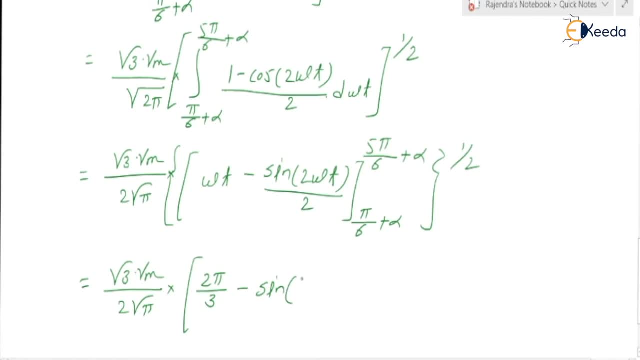 10 pi by 6. 10 pi by 6 is nothing but 5 pi by 3, okay, plus 2 alpha squared by 2: okay. plus can be written as sine of 2 pi by 6, that is a pi by 3 plus 2 alpha and pi by 3 squared by 2: right, the power 1. 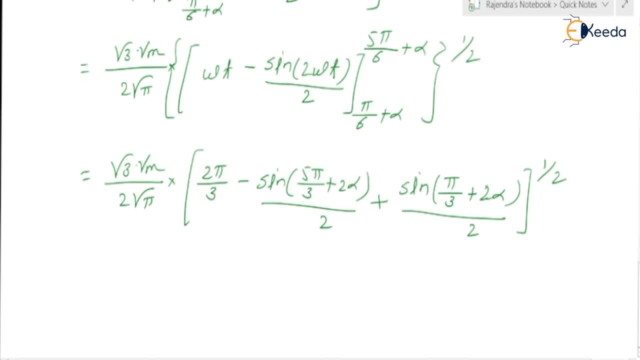 further. can we simplify it as sine of alpha plus beta. sine of alpha plus beta, yes, is equal to. we can write it as root: 3, 1 squared by 2 pi into 2, pi by 3 minus just 0.5, 1 by 2 into this can be written as sine of alpha plus beta, so it is sine of. 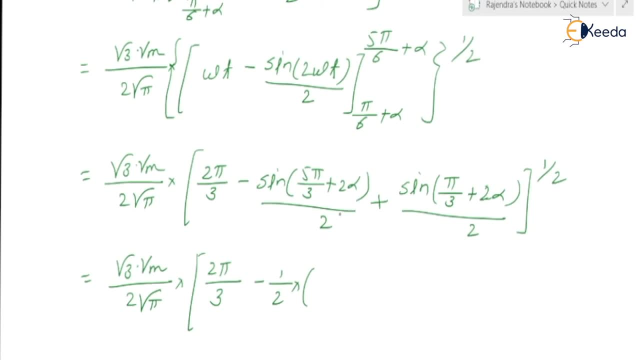 sine alpha, cos beta, right, plus cos alpha sine beta. okay, so pi into pi by 3 is a minus 0.86, right. so it is a minus 0.86 into cos of 2 alpha. next, it is a cos of 0.5. 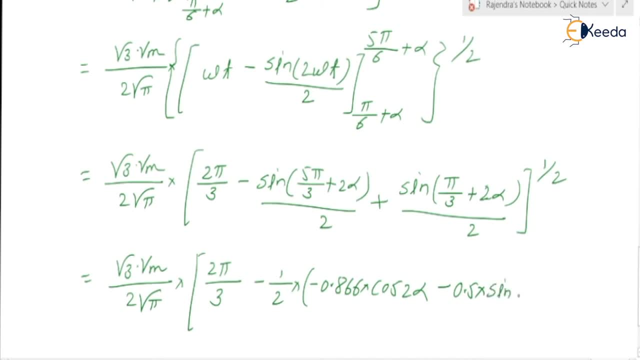 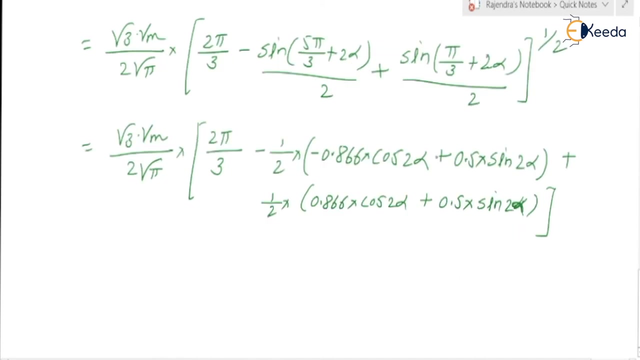 into sine of 12, the word term plus and write it as a by 2. into just sine of pi by 3, 0.866 point. into cos of 2, API, remove n. so if you check, yes, multiply with a minus so this term comes up again, otherwise på. 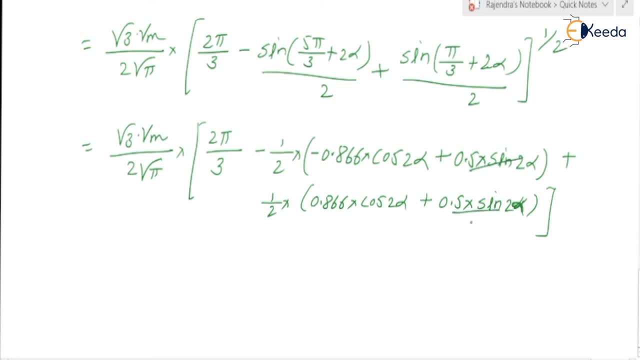 hereaver one. this is, if you remain okay, for society terms will get radish from. okay. what is this? be written as root 3 to vm, the power 1 by 2 divided by 2, root pi into: yes, this can be written as 2 pi by 3. this is minus minus. it will be plus okay and this plus okay. so it is a 0.866 into. 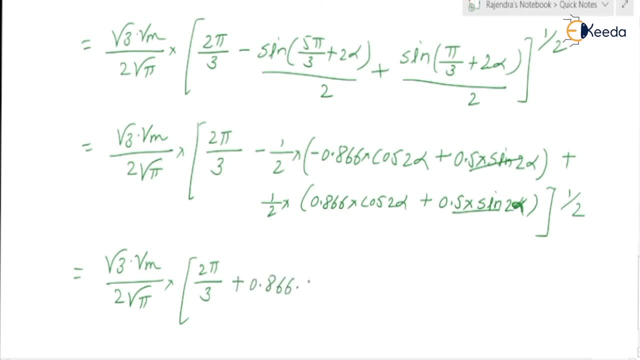 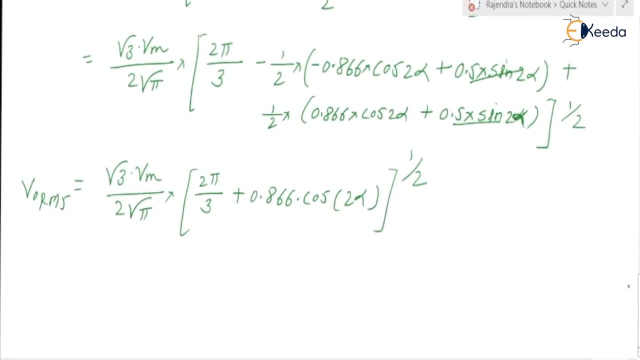 cos alpha plus, point into cos of 2 alpha, the power 1 by 2. okay, this is the expression of v0, rms, rm or alpha less than 30 degree, right alpha less than 30 degree, or less than or equal to 30 degree. is this clear? okay, we need to understand this expression. this is very, very important, okay. 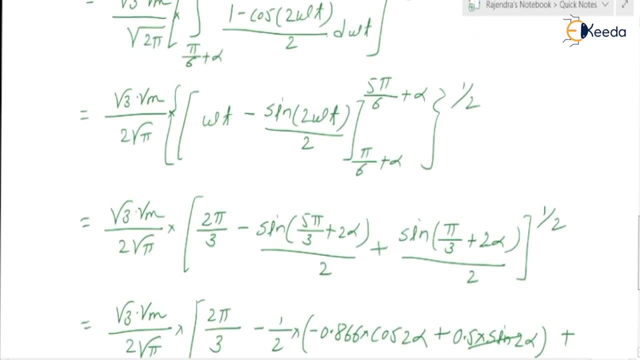 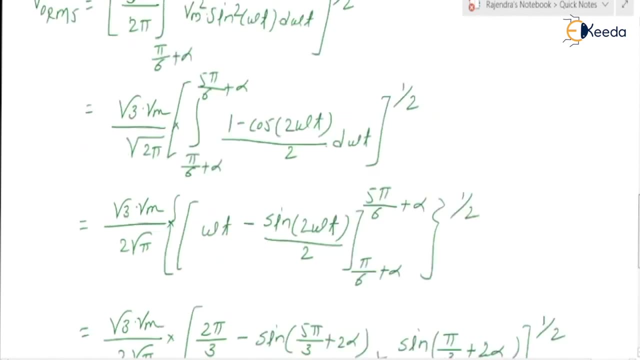 right: v0 average and v0 rms. okay, next, can we write the expression for or can we derive the expression for alpha greater than or equal to 30 degree? yes, we can simplify it for alpha greater than or equal to 30 degree. okay, so further for. 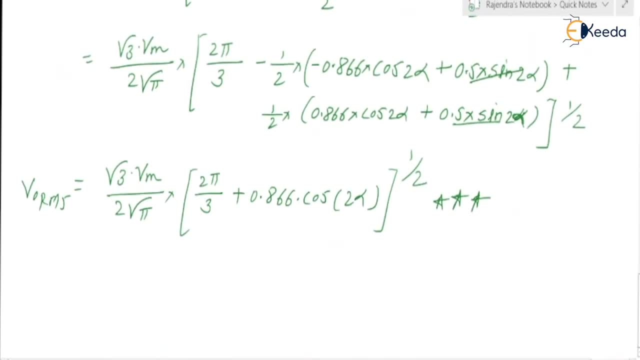 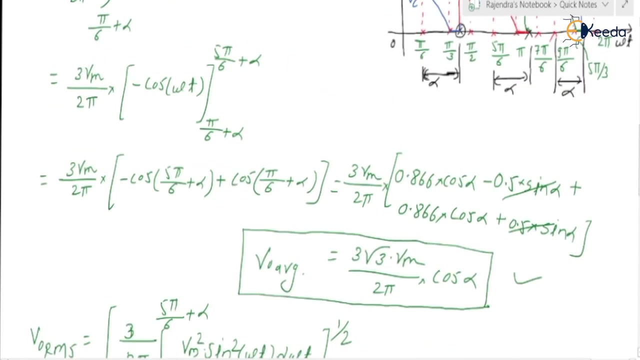 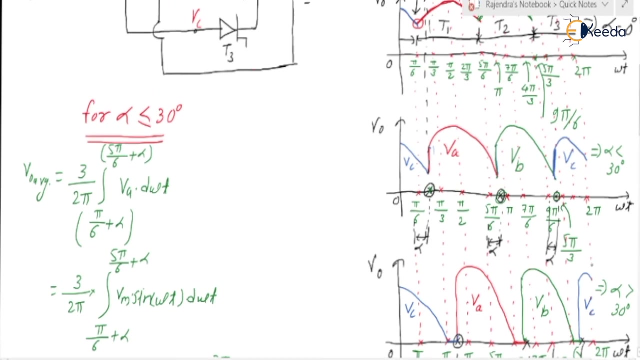 alpha greater than or equal to 30 degree- and i am continuing here- or alpha greater than or equal to 30 degree. so if you check the v0 waveform for alpha greater than or equal to 30 degree, yes, v0 waveform for alpha greater than or equal to 30 degree. right? so greater than 30 degree. this. 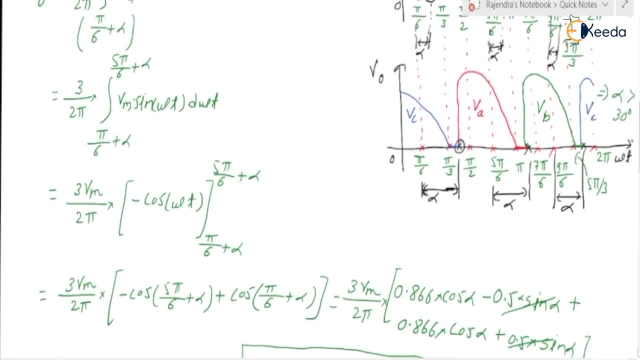 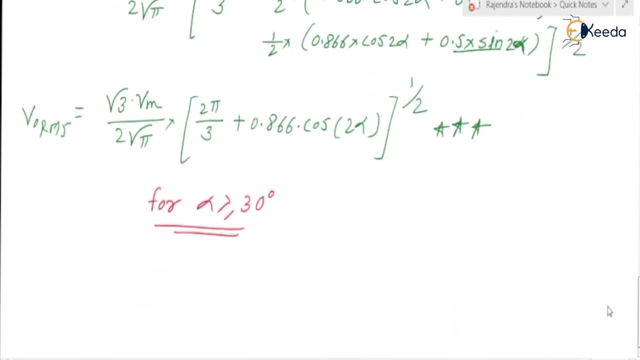 is the waveform okay. so if you check in this waveform, yes, the va is appearing from pi by 6 plus alpha till pi only. okay, so upper limit should be pi right. upper limit should be pi right, because after pi the output voltage is zero, right? so here we can write v0 average. v0 average equal to. 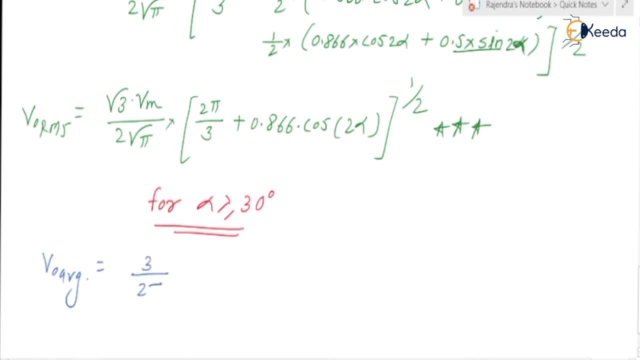 three by two pi, right, three by pi. okay. integration from pi by six plus alpha to yes pi. okay, it is a v a v. a. is vm into sine of omega t, into d omega t, right? so further can we simplify it as: yes, 3 vm by 2 pi, 3 vm divided by 2 pi into yes, integration of sine. it is a. 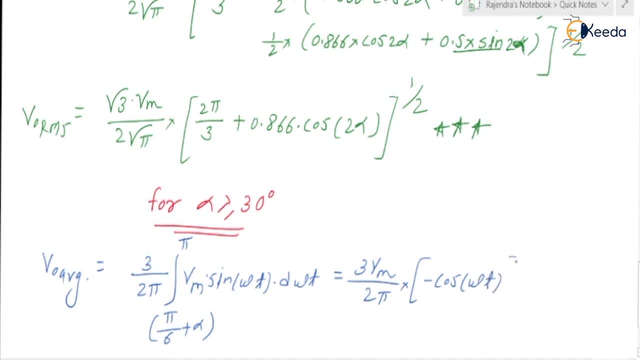 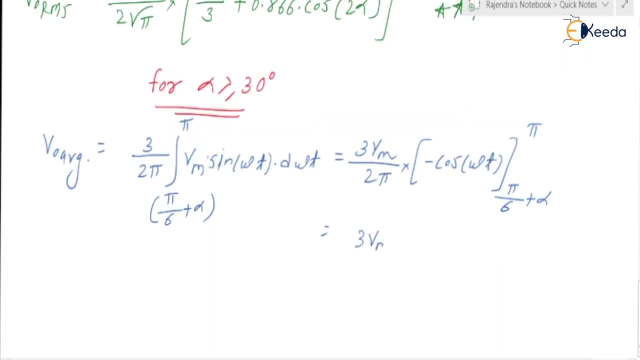 minus cos of omega t to the limit pi by 6 plus alpha 2 pi. okay, so this can be written as: is equal to: yes, it is a 3 vm by 2 pi is equal to dm divided by 2 pi. okay, into yes minus cos of omega t. okay, so this can be written as: 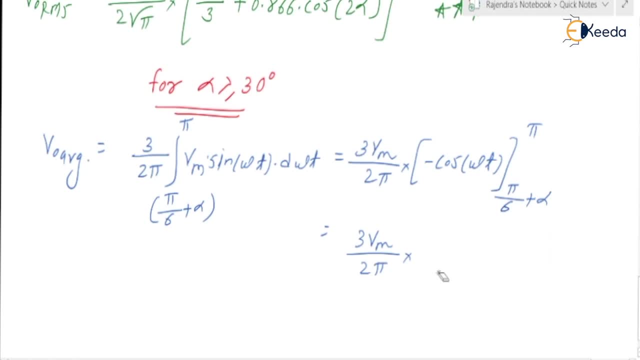 What is the cos of minus cos of pi? right, putting the limit right so we can write it as a. yes, we can write it as a minus cos of pi. cos pi is minus 1, so it is a 1, okay. plus cos of pi by 6 plus alpha: okay, this is the Wieser average for alpha greater than or equal to 30,. right, no need to expand this term. okay, keep it as it is. okay, keep it as it is. 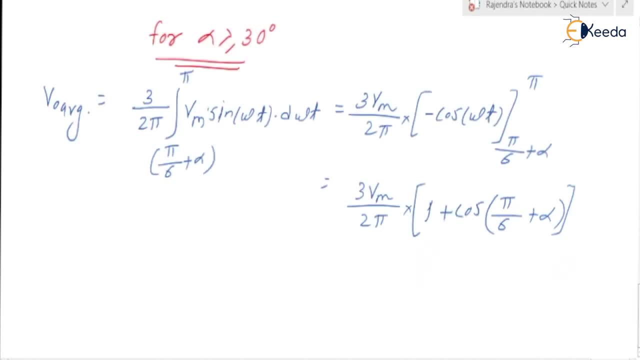 Next, V0 RMS right. V0 RMS for alpha greater than or equal to 30 degree. okay, so it is again 3 by 2 pi right integration from pi by 6 plus alpha right 2 pi. okay, is the Vm square to sin square of omega t into d omega t, okay. 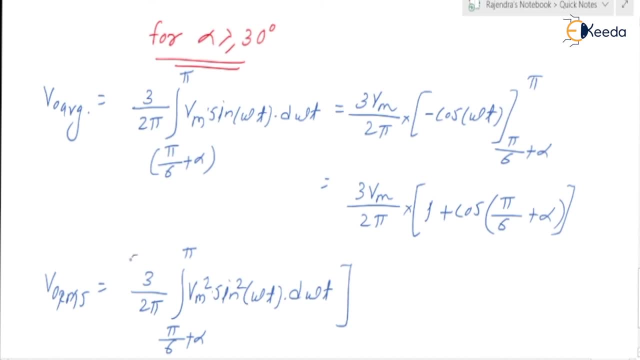 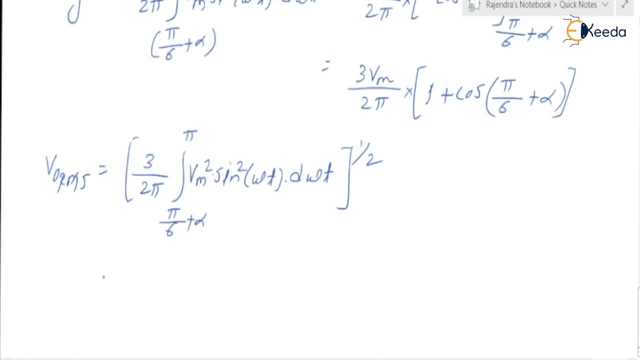 so which is equal to or to the power 1 by 2, right that we need to write okay. so further we can write it as is Vm upon root 3 into Vm upon root 2. pi okay into yes. integration from pi by 6 plus alpha to pi: yes. pi by 6 plus alpha to pi: yes. 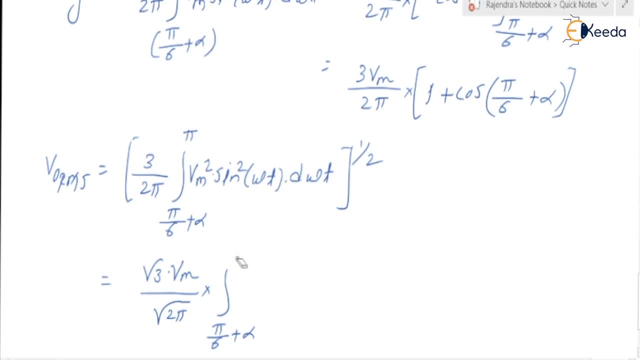 okay, And we replace sin square of omega t theta 1 minus cos of 2 omega t less 1 minus cos of 2 omega t. third power 2 to d omega t, the power 1, right, okay, Next further, can we write it as yes is equal to root 3 into Vm. 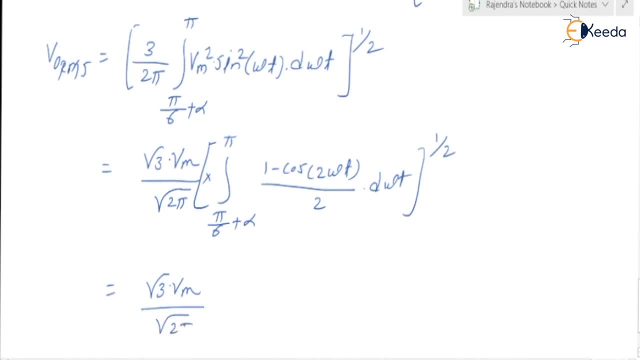 by root 2 pi. or can we take this 2 outside? Yes, so it will become 2 root pi. right, So this term will become 2 root equal to further, we can write it as a omega t and as integration of pass. it is sine of. 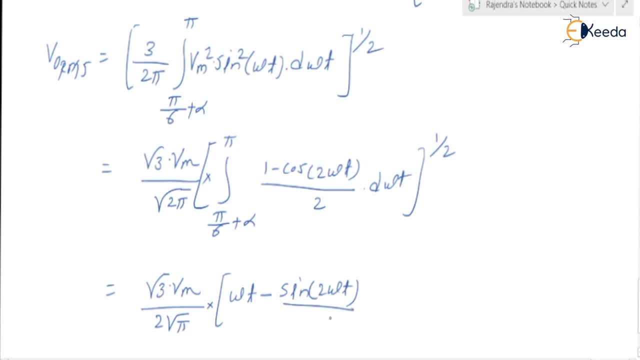 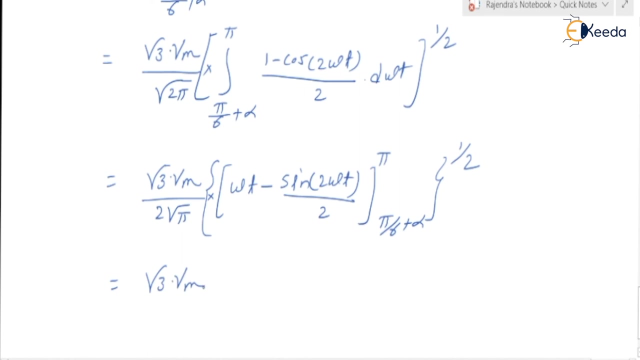 2 omega t divided by 2, mid pi by 6 plus alpha pi, okay The power 1 by 2. So again we can simplify it as equal to s root 3 into vm. divided by pi into s is a pi minus pi by 6 minus alpha.